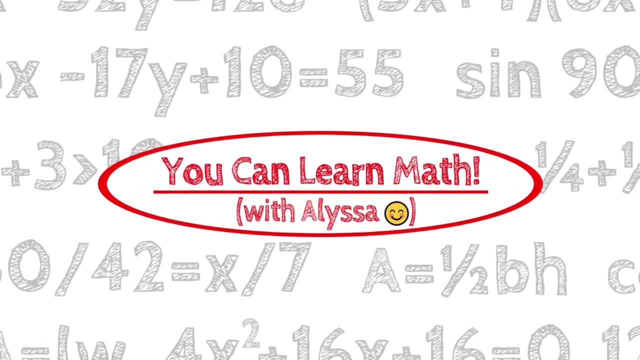 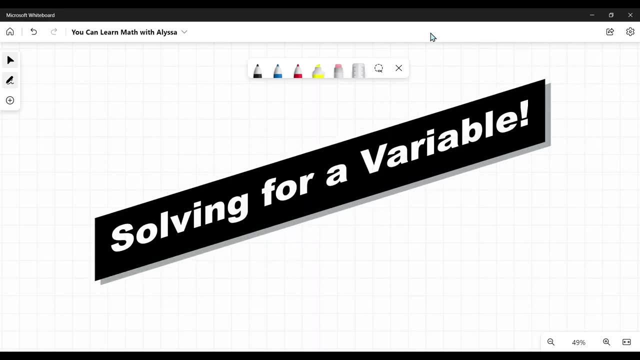 Hi everyone. it's Alyssa and welcome to. You Can Learn Math. Today we're talking about solving for a variable. Notice, I'm not saying solving for x. That is a different connotation. That usually means we're doing something like 3x equals 15.. What is x? 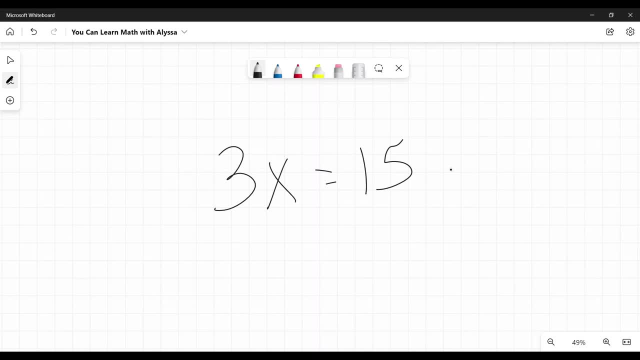 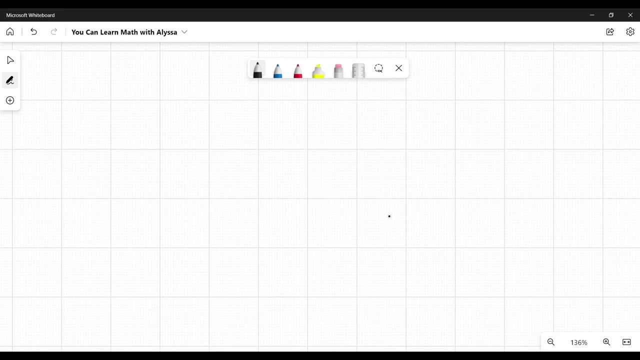 What is the value of x? Whenever you hear solve for x, that's generally what we're talking about. There are exceptions, of course, but general rule. we're talking about finding the value of something If it's solving for a more generic variable. when you get to this part of your math, 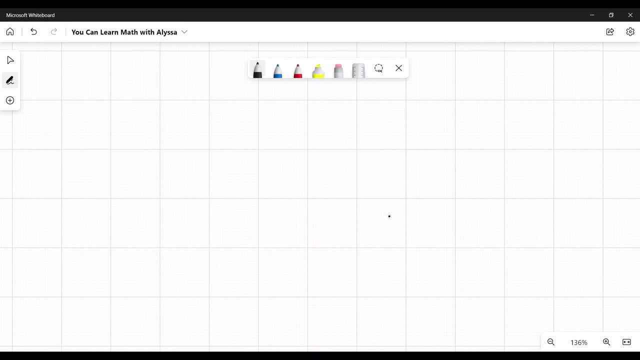 book where it says: solve for a variable totally different thing. And we kind of have to push that. we're trying to figure out that x equals a number. What is that number? That's not what we're talking about. That's not what we're talking about. That's not what we're talking about. 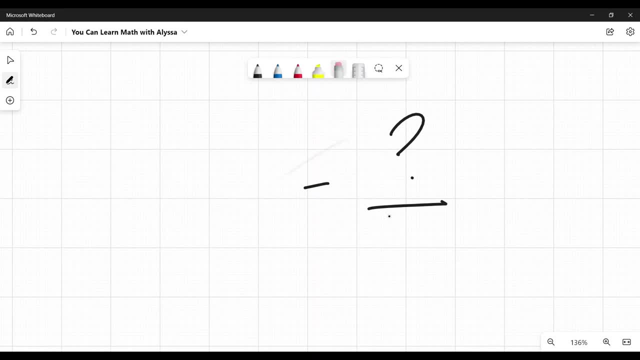 We're going to be doing here and it can be hard to get out of that mindset With these problems. you're going to see a ton of variables and they differ wildly and they don't really mean anything. For example, it might be x equals w, y, z. 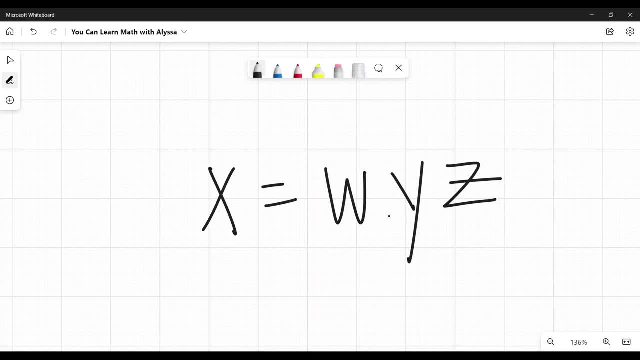 and you're told to solve for y, But there's no numbers, How can I tell you what y is? And this is where we have to get out of that mindset. We are not figuring out the value of y as in a specific number. When you see this solve for a variable, what I want you to think is: I want that variable. 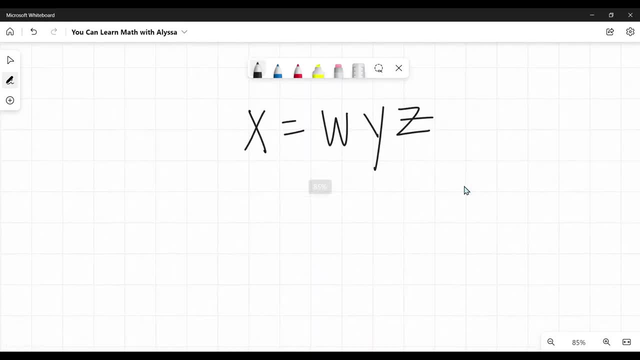 to be all by its little lonesome and everything else to be on the other side. So your answer is going to be: y equals something, We don't know what yet. but when it says solve for y, your answer better have that variable. 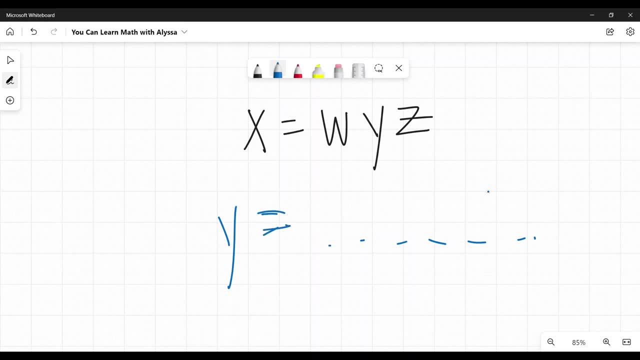 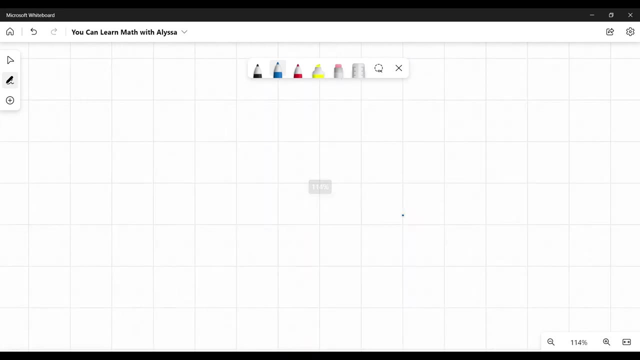 In this case, y by itself equals and everything else in the problem needs to be over here on the other side, And these come in a variety. They get more complicated as they go. So let's start with a more basic or introductory one And let's say that it is: y equals six times s, and they say to: 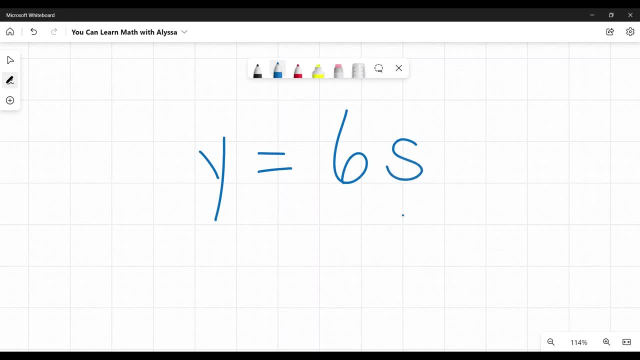 solve for s. So what we're going to think about is we're going to look at which side s is. It's over here on the right, And I want to get rid of everything that isn't s. Everything that isn't s needs to go over here. 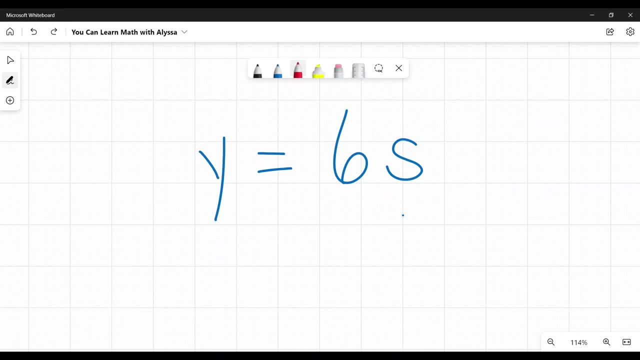 And I need to figure out how to do that. So for this, I find it's most useful to think of undoing what's been done to s, And we want to undo it. We want to go backwards like in reverse order. 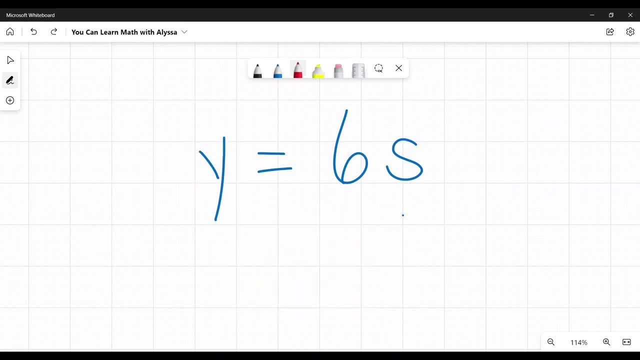 So in this case I'm not really concerned with what's on the left just yet. I'm just looking at the side with s. What's been done to s? This means six times s. s has been multiplied by six. That's it. Nothing else has. 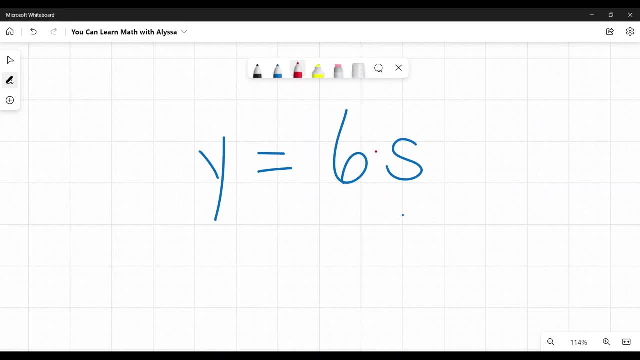 happened. I want to undo that. So what's the opposite of multiplying by six, Dividing by six? So I'm going to divide both sides by six. So on the right hand side, since I've multiplied by six and then divided by six, that's undone it. 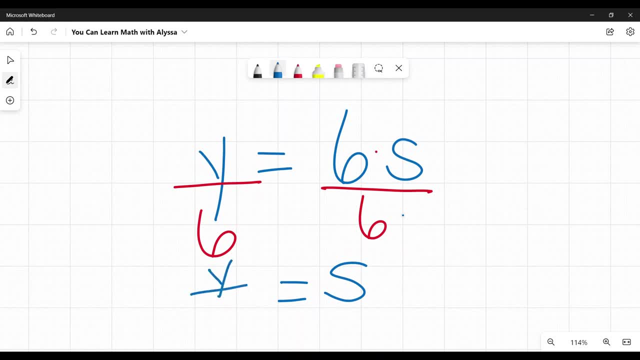 So s is by itself, And on the left hand side I have y divided by six, And that's it I've solved for s. s is by itself over here. Everything else is over on the left, And that's that's the goal. 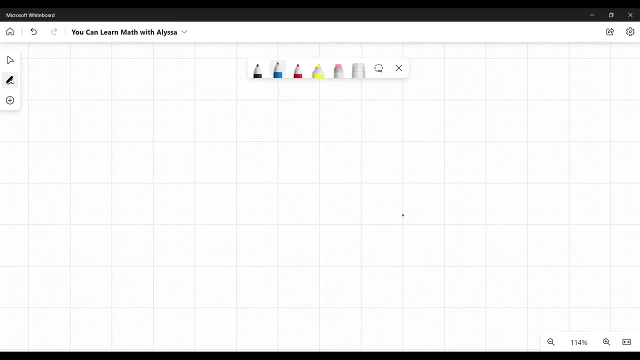 That's what we're wanting. So each one of these, we're going to be just undoing what's been done And they're going to start out with more straightforward or one step versions of this. For example, they might say: z plus four equals t, Solve for z. Again, I don't really look at what's on the right hand. 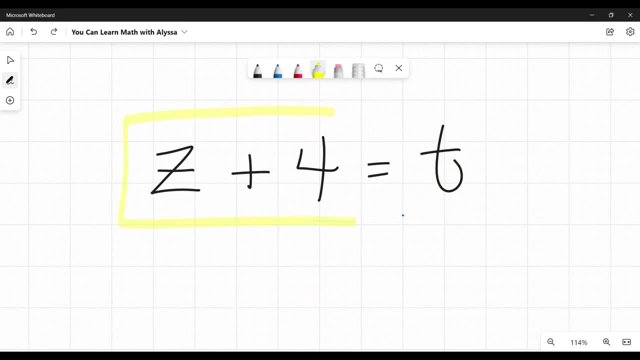 side just yet. That doesn't matter for my plan of what I'm going to do. I look at the side with z And I go. what happened to z? Four was added to it, So I need to undo that. What is the opposite? 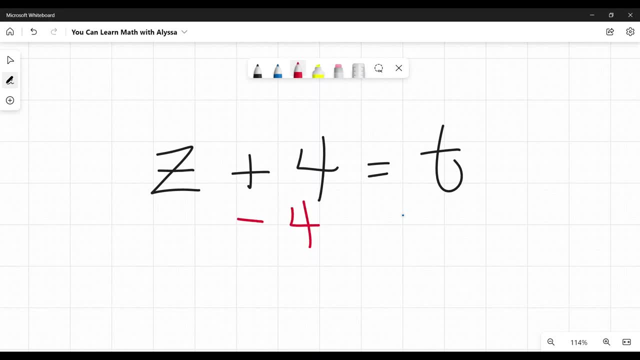 of adding four, It's subtracting four. Now, in algebra, just as a reminder, every time there's an equal sign, an equation, it's like a, like a seesaw, And you've got two perfectly balanced people sitting on this seesaw. And if I want that seesaw to stay perfectly balanced, whatever I do to, 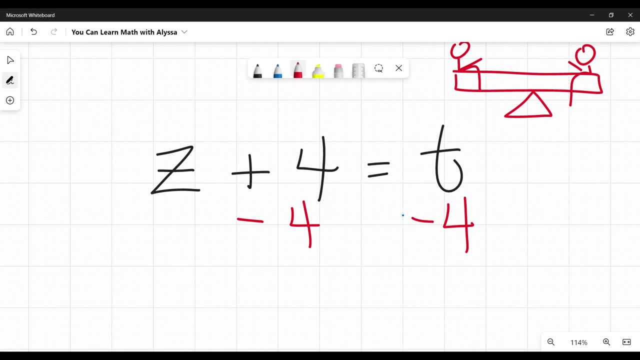 the left side I have to do to the right. So that's why here I subtract four from the left. I have to subtract four from the right, So it still stays equal and balanced. Now that I've added four and subtracted four, that undoes what's been done to z. So now z is by itself. 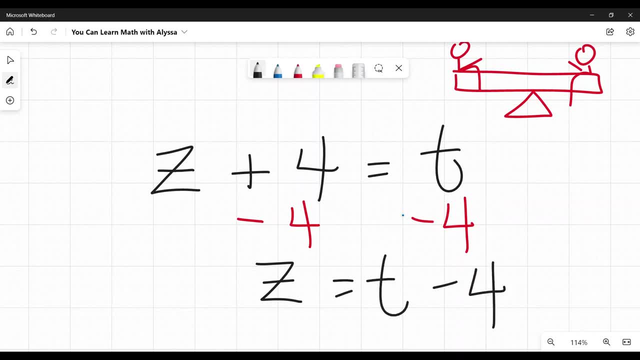 And on the right I have t minus four and I have solved for z. Now, as you might guess, it doesn't stay this straightforward and one step for very long, Pretty quickly, they're going to add some extra wrinkles to it And they're going to add more. 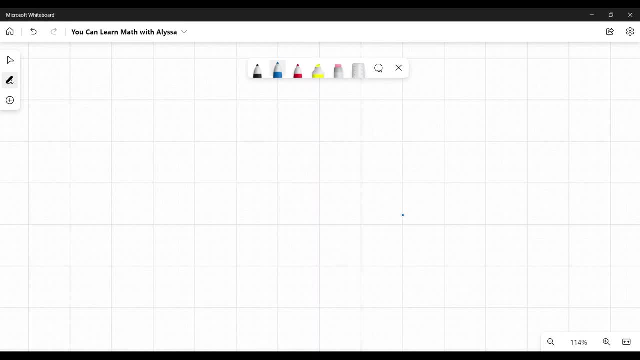 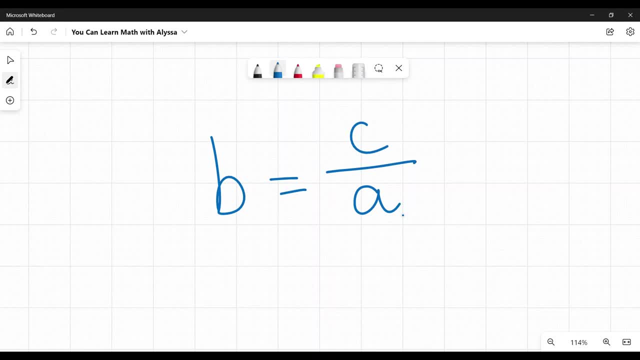 Let's say that I've been dividing, multiplying, adding, subtracting previously. It's just all variables. The same rules apply. I want to solve for c. So what's been done to c? C has been divided by a. What's the opposite of dividing by something? Multiplying by something? 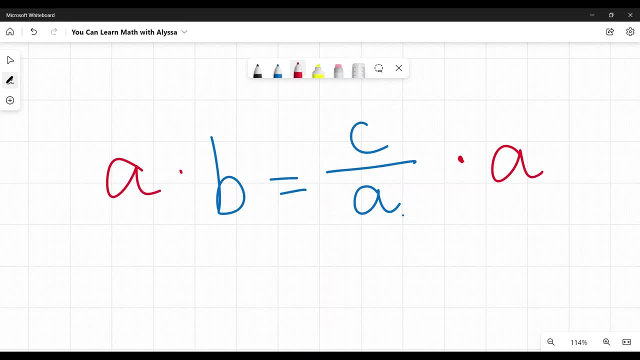 So I'm going to multiply both sides by a, C being divided by a and then multiplied by a. that undoes that division to multiply by a. So on the right right I just have C and on the left I have A times B, and I've solved for C. Well, let's add. 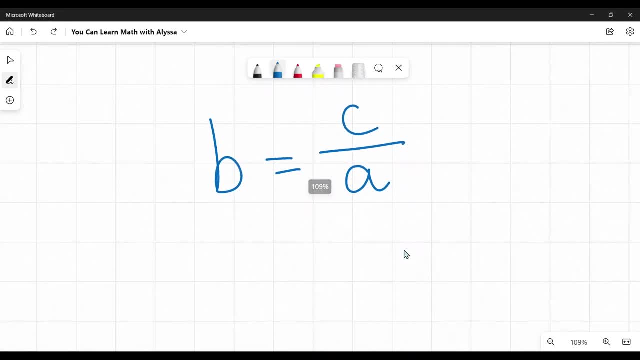 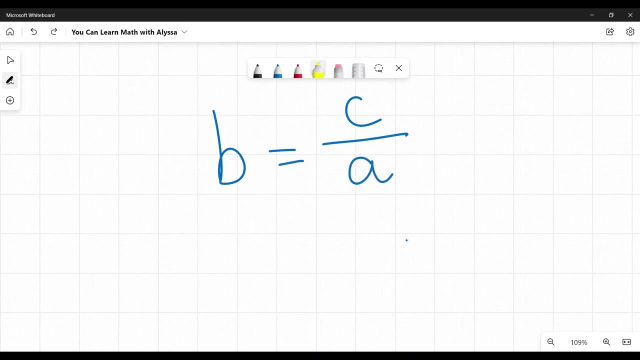 a little wrinkle to this. Let's say we started at the same point, but instead of solving for C, they said no, solve for A. Ooh well, how do I do that? Because A hasn't had anything done to it. 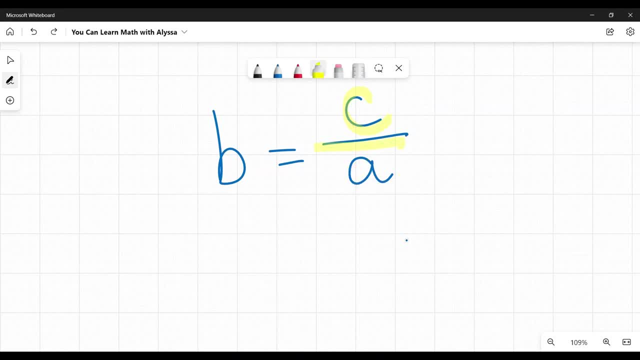 C has. C was divided by A, So it's not A being divided by C, So I can't undo that. What do I do This? we have to get it. We have to work with it a little bit to try to get A in a position where 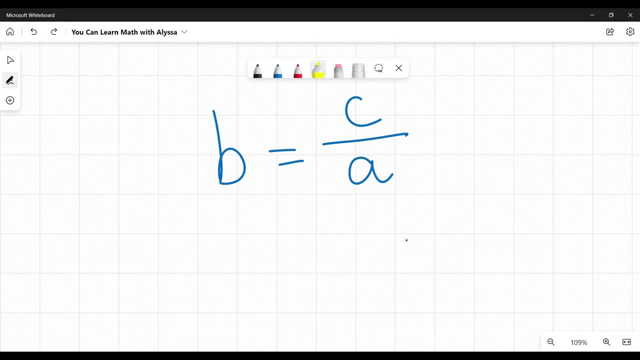 it can be by itself or something's being done to A that can be undone. So this sort of scenario- this is a very common one, you're going to see. The first thing you want to do is: we want to get A over to the side, Basically do. 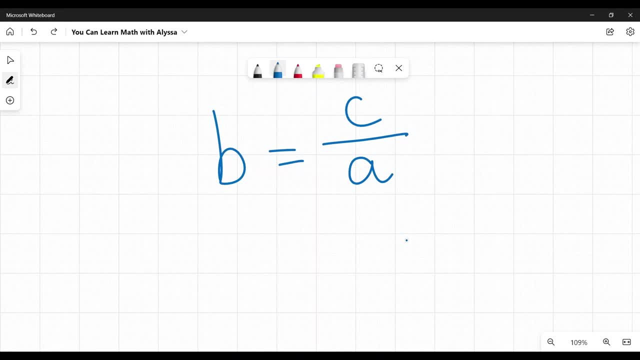 what we just did, but that's just the first step, So okay. So I'm going to like we did before. I'm going to multiply both sides by A, and that gives me A times B equals C, like we just saw. 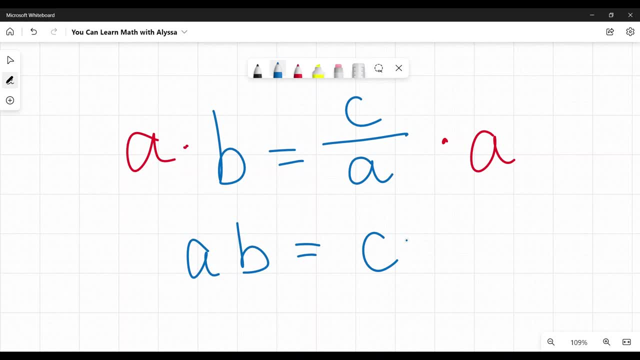 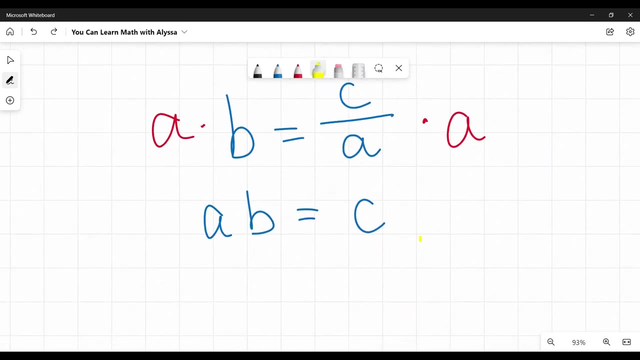 in the previous example. So A times B equals C. Well now, now we're in a position where something is being done to A. A is being multiplied by B, So now I can undo what's been done to A, So A is being multiplied by B. What's the opposite of being multiplied by B Being divided by B? 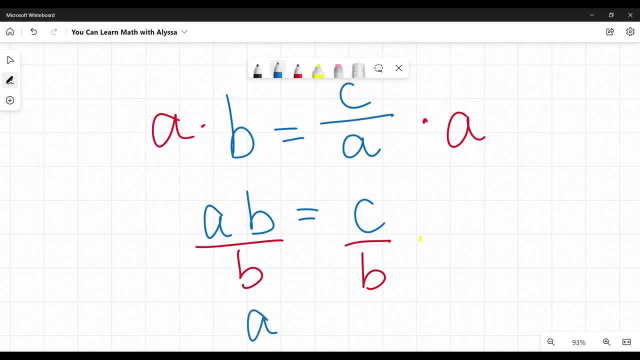 Now that undoes what's being done to A, And so A equals C divided by B, And that would be my final answer. They also like to do things where they combine multiplication, division, subtraction, addition. They love adding things in there. For example, it might be A times. 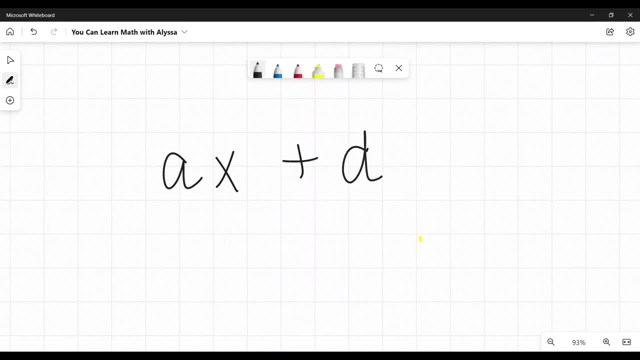 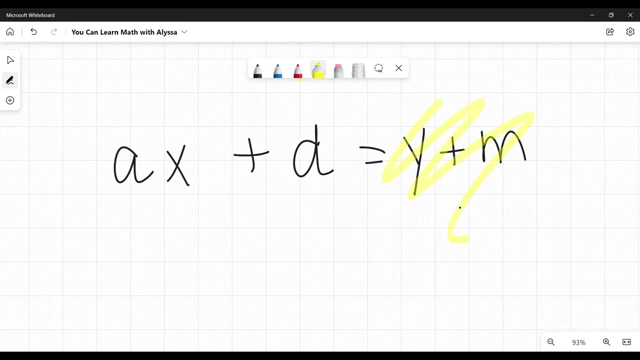 B times B, O times B. X plus D equals Y plus I don't know M. Let's say they said I want to solve for X. Okay, So now this point, this part doesn't matter, The Y plus M, it doesn't really matter. 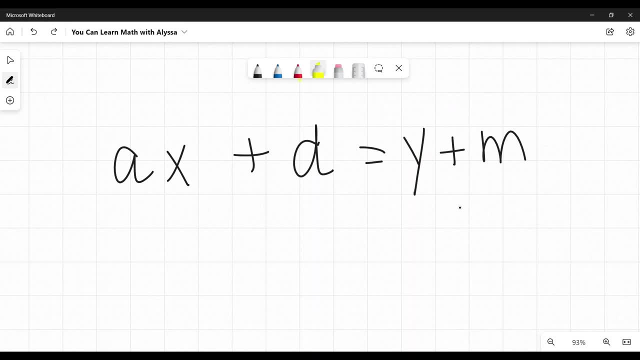 So I'm going to look over here What's been done to X And we want to go in order and then go back back back in reverse order. So x has been multiplied by a. that was the first thing that happened to x. 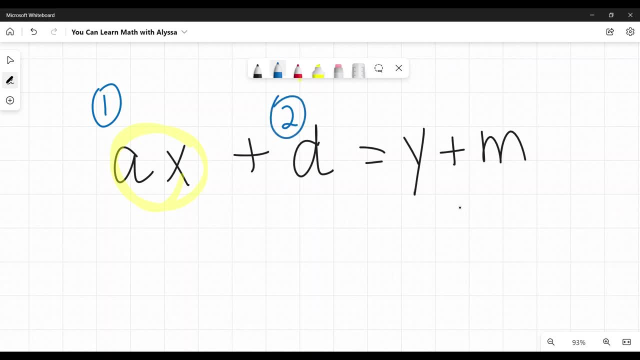 The second thing was d was added to it. So this was the first, this is the second. We want to go backwards in reverse order, so we want to undo the second one first and then undo the first one. To add d. the opposite of that is to subtract d. so I'm going to subtract d from both sides. 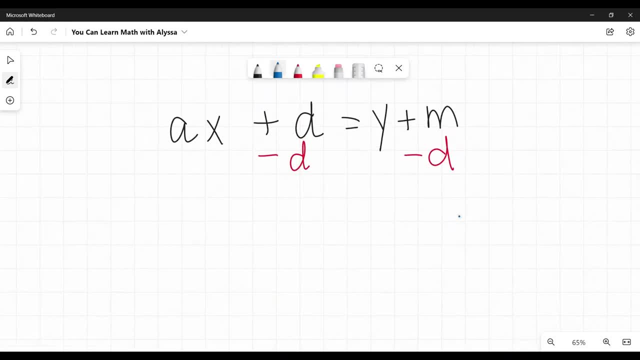 I'm going to zoom out a little bit and move up here, And so that gives me a times x on the left equals y plus m minus d on the right. Now this next step. be careful on this one and also make sure you know how your teacher 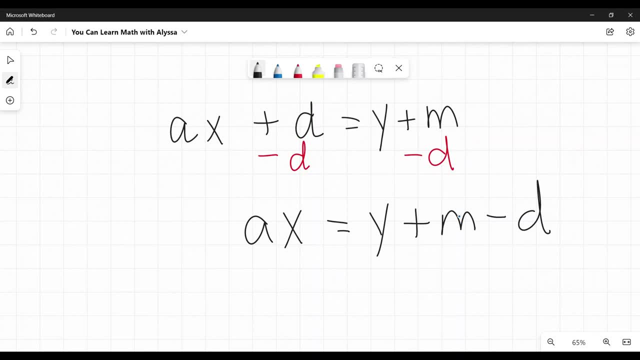 wants you to present the final answer. more on that in a second. The next thing we're going to look at is: okay, what's the other thing that happened to x? It was multiplied by a. We want to undo that. so we want to divide by a. 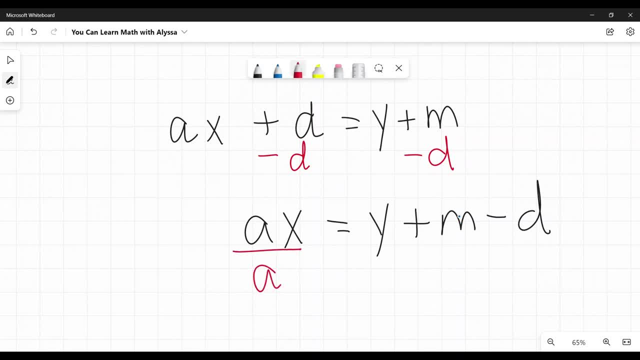 Now here's the part to be a little careful. There's two different ways you can write this. They both mean the same thing, but if the directions or your teacher are saying: present it this way, please present it the way they want you to. 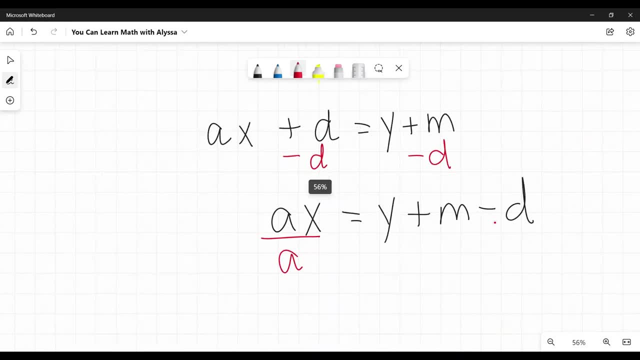 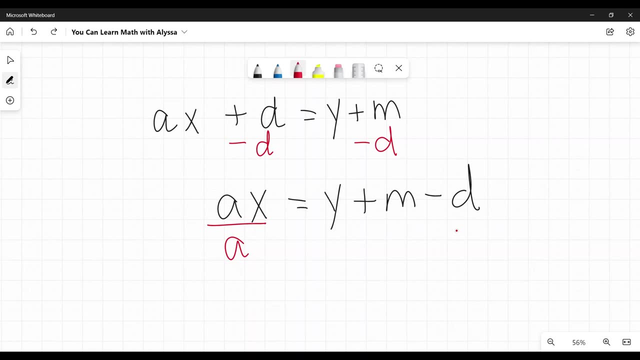 We don't want you to lose points on a technicality here. So the two ways that this might be presented: when you have a long string of things that's being divided by a single number, It may be written as y plus m, minus d, all over a, or you can put each one over a. 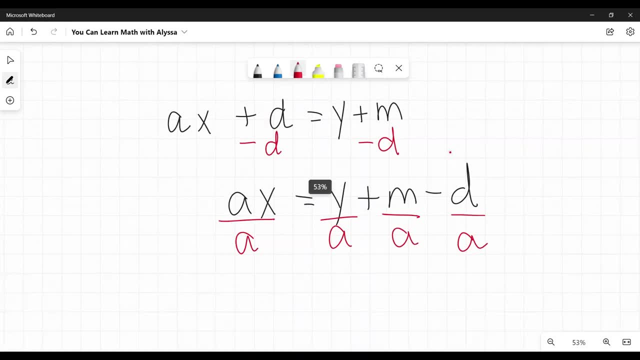 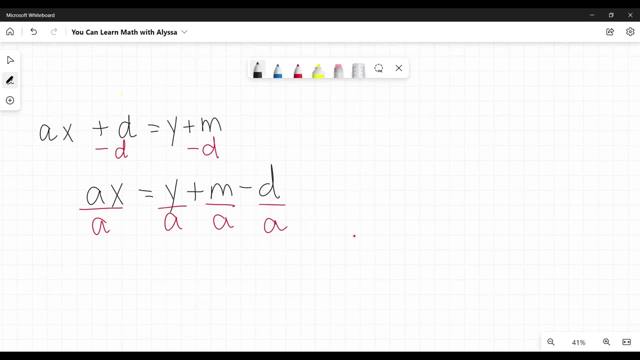 It literally means the same thing. As a little side note, the reason: it means the same thing. if you put some real numbers in there it'll help. you see it Like, let's say I said two fifths plus three-fifths.